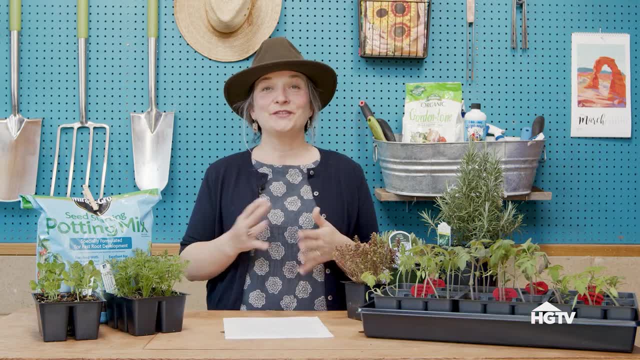 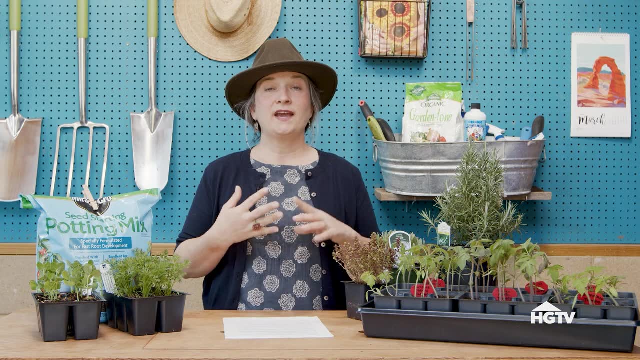 Alaya asks: can you plant herbs all in one pot? If you're looking to grow some of the most common herbs, it's important to know first what season they grow best in- whether they're annuals or perennials, and what kind of soil and water conditions they like. Not all herbs are the same. 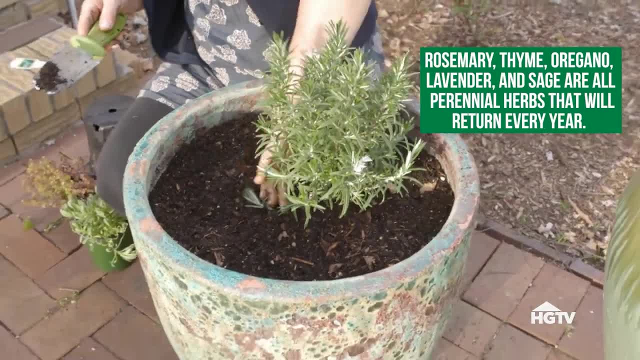 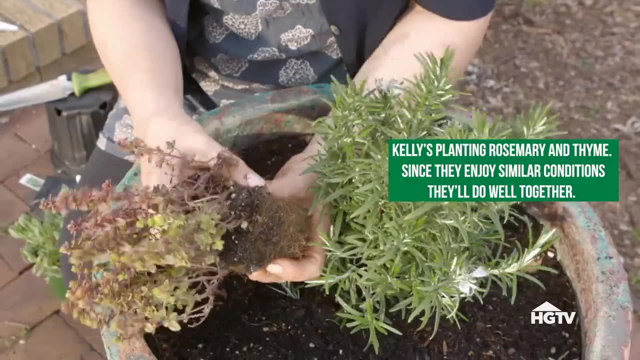 Rosemary, thyme, oregano, lavender and sage are all perennial herbs that like drier soil conditions because they're originally from the Mediterranean climate. You can plant those together and they'll come back year after year. Just be sure to look at spacing recommendations. 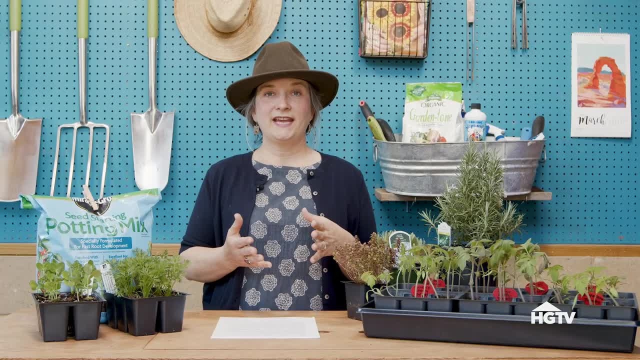 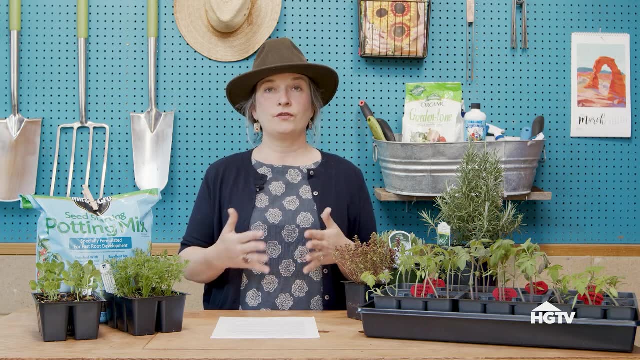 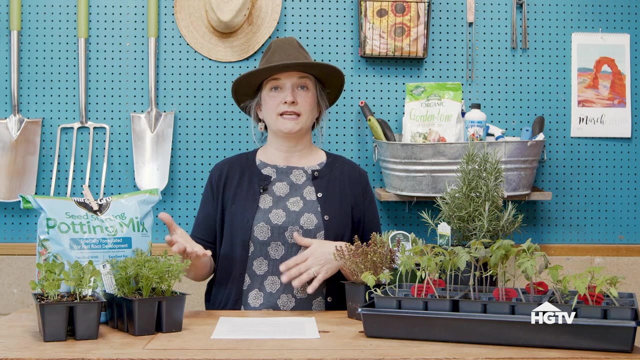 as some of these can get quite large. On the other hand, basil, dill, cilantro and parsley are all annuals that like a good amount of water, so you could grow those together. Cilantro and parsley like cooler weather, while basil and dill are more summer plants. They like the heat. Mint is kind of. 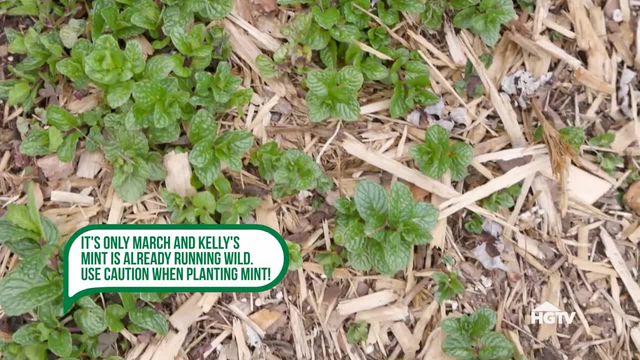 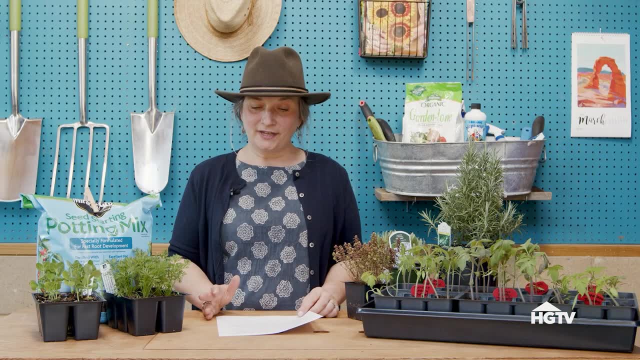 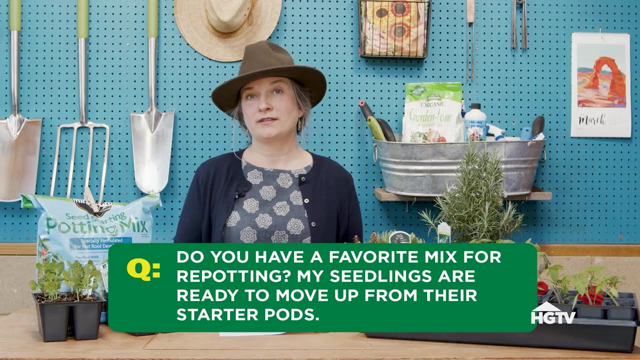 in its own category. It will come back year after year, but it will also spread a lot and take over the plant mint in a pot by itself. Josh is starting his summer plants from seed indoors and asked: do you have a favorite mix for repotting? My seedlings are ready to move up from their starter. 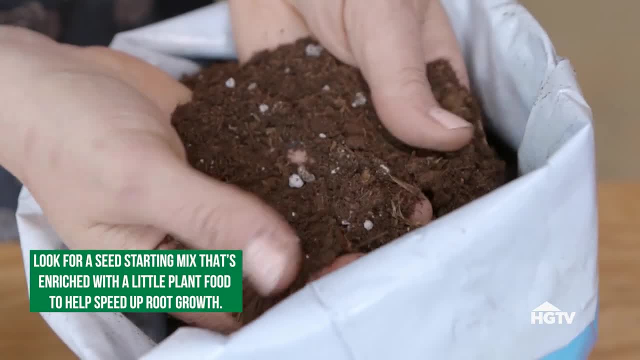 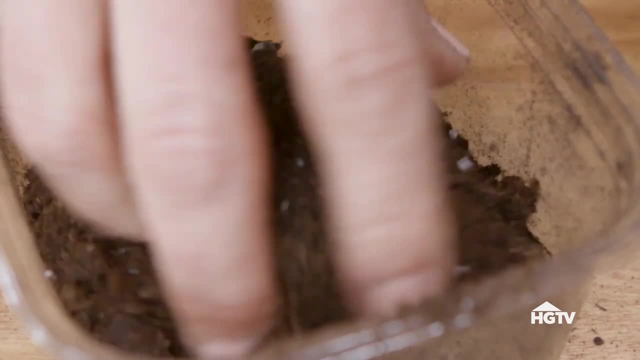 pots. I've recently been using this seed starting potting mix and I like it a lot. I wasn't sure at first because it does have larger chunks of organic material than I'm used to in a seed starting mix, but it seems to hold water really well and not dry out as quickly as other mixes. 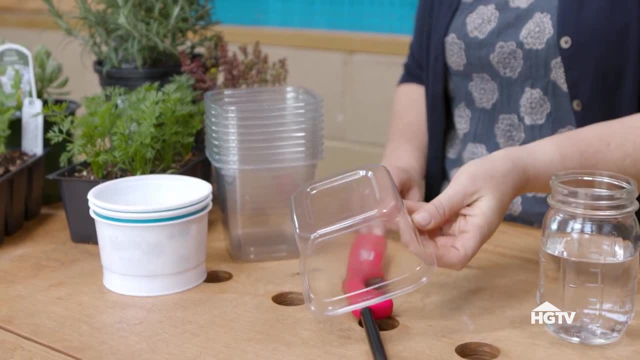 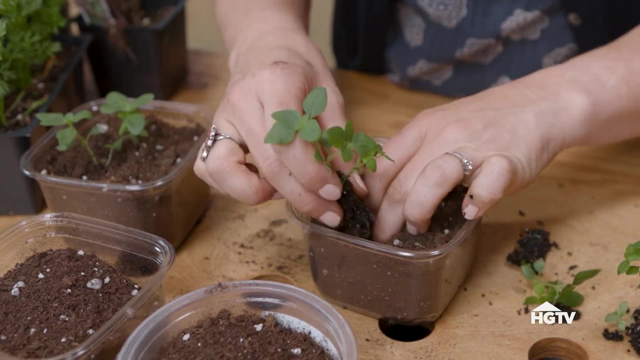 I'm stepping up some of my seedlings into larger pots too. I've been using plastic containers to reuse for potting, so I'm not wasting so much plastic. If you try this too, just be sure to poke lots of holes in the bottom for good drainage. Now I want to show you. 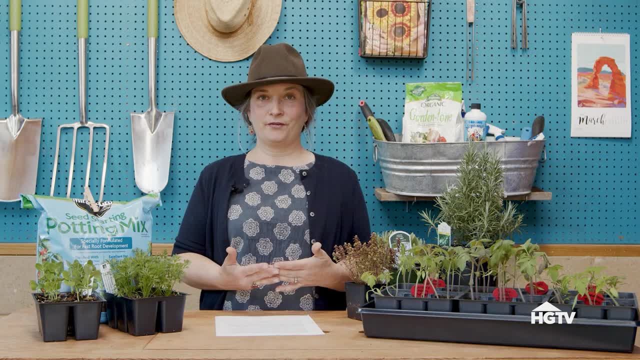 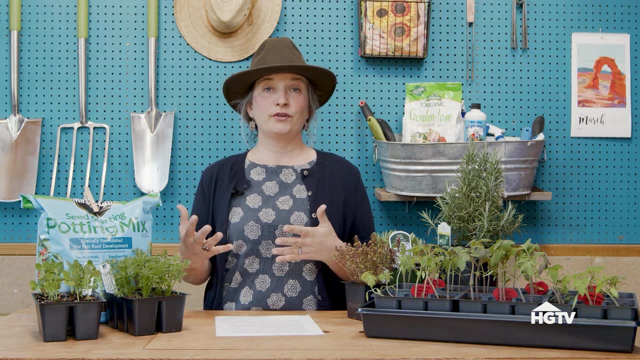 a little problem in my garden. Brussels sprouts are a bit of an experiment for me. In my warmer zone, in zone seven, you should be able to plant them in fall and keep them alive through the winter and then have them produce in late winter or early spring. So I've been using row cover on. 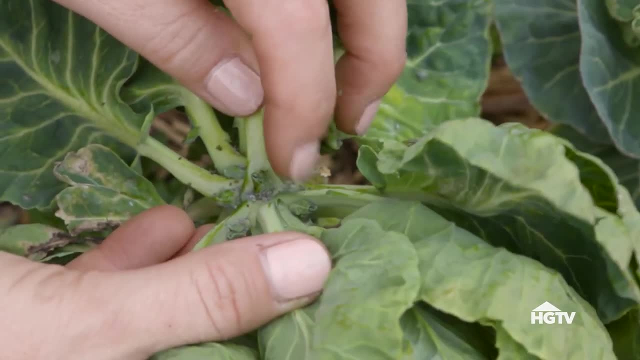 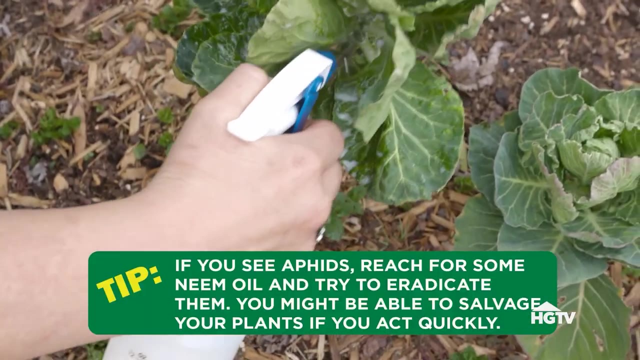 cold nights and keeping them alive, but they're not really thriving. I just spotted aphids on the sprouts of a few of the plants. That's a sign that they're not super healthy. but I'm not going to pull them up just yet. I'm going to knock the aphids off the best.